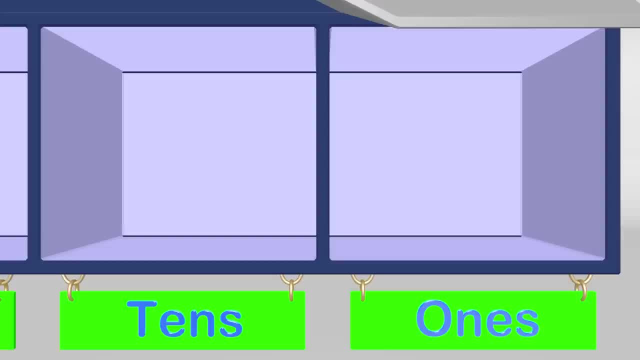 There are rules in this house that have to be followed, And one of the rules is that you can only have one digit in each room. A digit is any number from 0 to 9.. Let me show you what I mean. Here is the number 2, and this is one digit, because there is just one number. 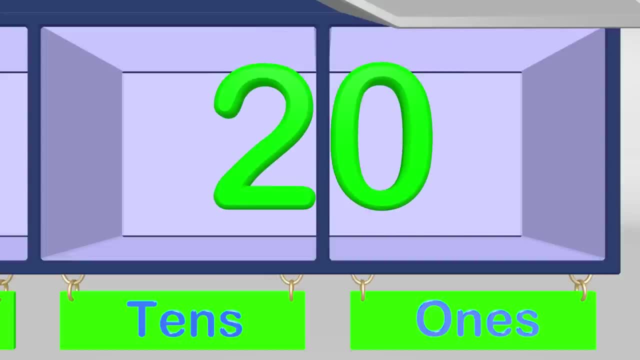 Let's look at another number. This is the number 20.. Can you tell me if this number has more than one digit? Yes, the number 20 has two digits, because the 2 is a digit and the 0 is a digit. 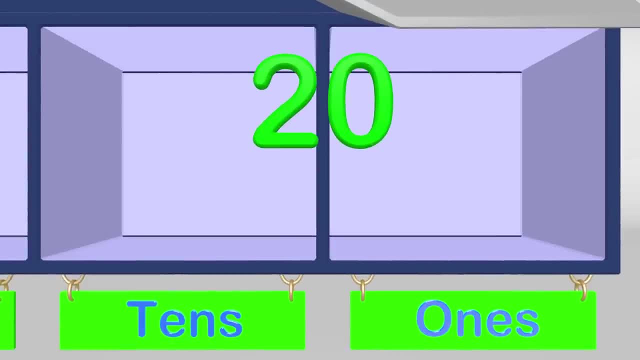 Uh oh, we cannot put both numbers in the ones room. We have to split them into each place. This is still the number 20.. We just have the 2 in the tens place and the 0 in the ones place. Now that we have that rule out of the way, let's look at some place value blocks. 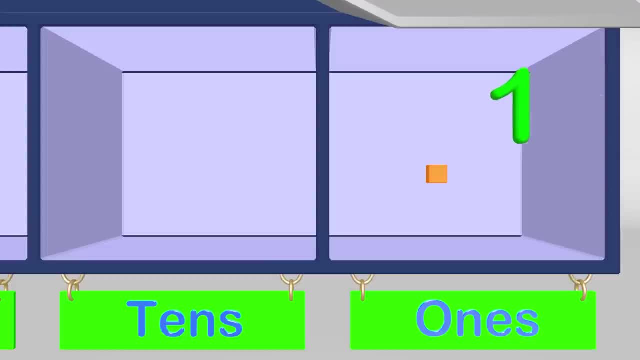 Here is a ones block. This ones block is worth 1 and is represented by the number 1.. What if I add more ones blocks to the ones place? How many ones blocks do I have now? I have 5 ones blocks, Great job. 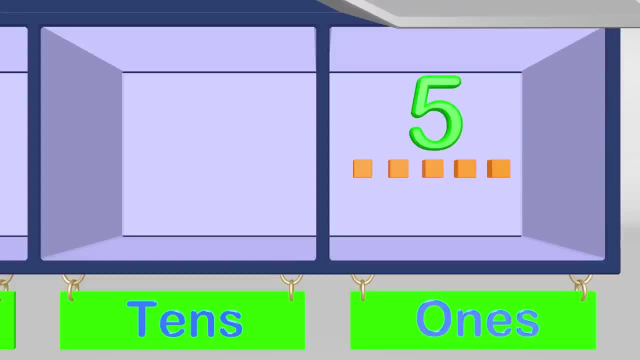 We can see the number 5 above the room and we are not breaking the house rules because we still have just one digit in the room. Now let's add 4, more ones blocks. How many blocks do we have now? Can you count them for me? 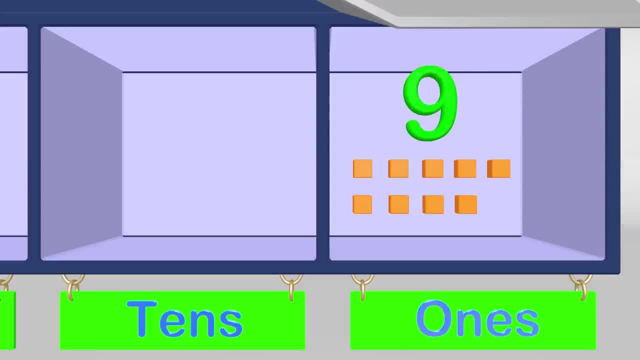 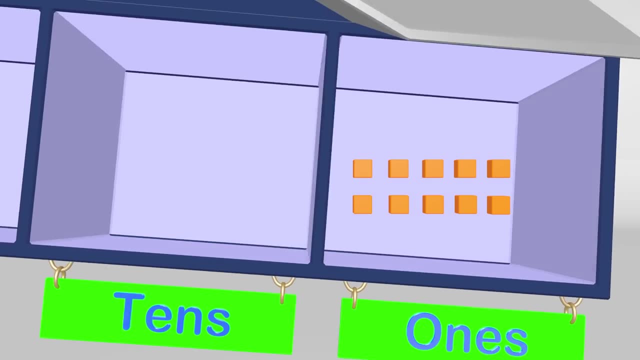 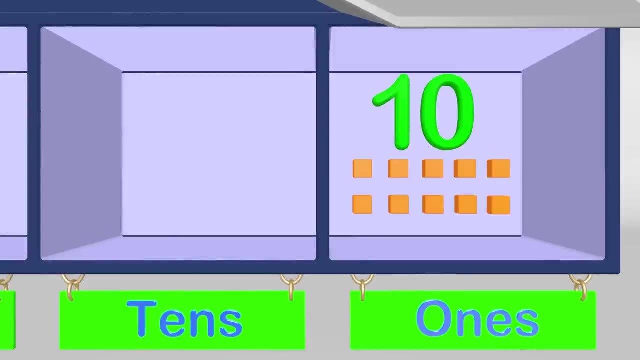 We have 9 of the ones blocks. Great job again. But wait a minute. another block just moved into the ones place, but something is wrong. I think I know what it is: We have reached the number 10.. Because we have reached the number 10, we have more than one digit and we are breaking the rule of one digit per room. 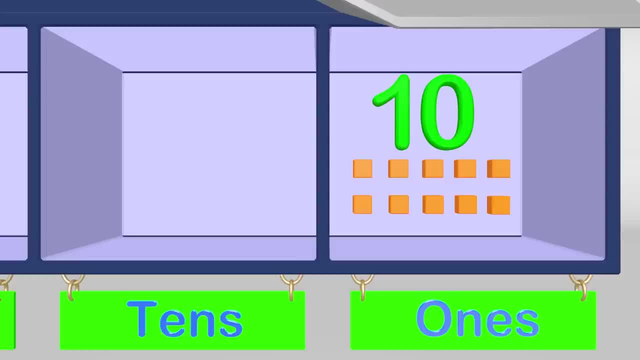 Now here is the really cool part that I learned the other day. Watch what happens to the blocks when there are 10 of them in the ones place. All of the 10 ones- blocks stuck together to form what we call a tens block. This is a group of 10 ones called a 10.. 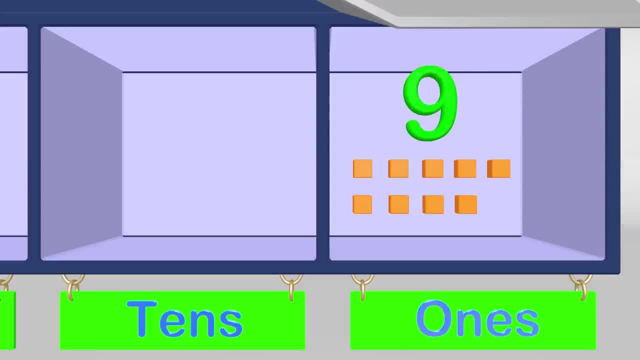 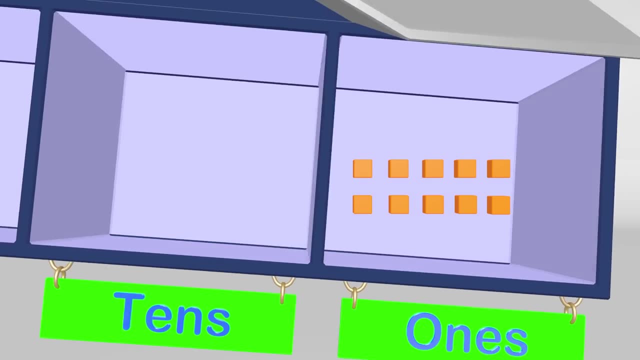 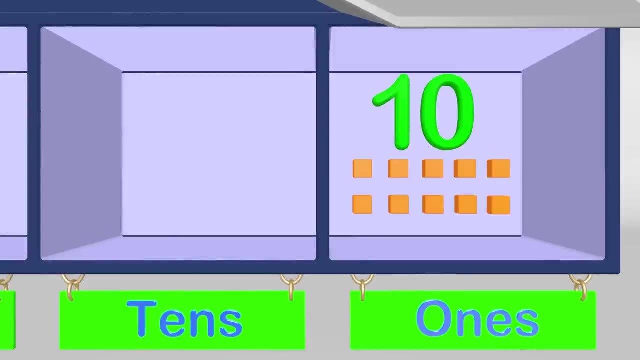 We have 9 of the ones blocks. Great job again. But wait a minute. another block just moved into the ones place, but something is wrong. I think I know what it is: We have reached the number 10.. Because we have reached the number 10, we have more than one digit and we are breaking the rule of one digit per room. 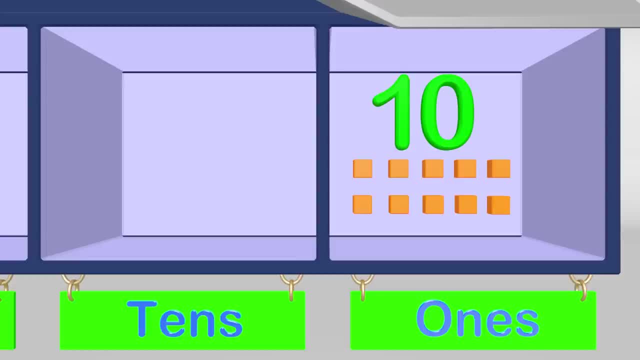 Now here is the really cool part that I learned the other day. Watch what happens to the blocks when there are 10 of them in the ones place. All of the 10 ones blocks stuck together to form what we call a 10s block. 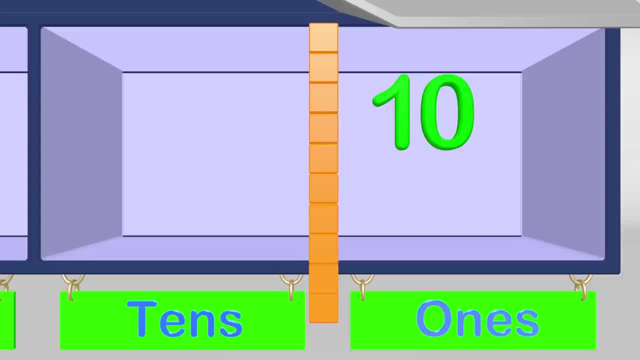 This is a group of 10 ones called a 10.. Why do you think we call this a 10?? We call it a 10 because this 10s block is made up of 10 ones blocks. You guys are awesome. When we had 9 of the ones blocks in the room, we had no problems, but once we reached 10, we had to form a 10s block. 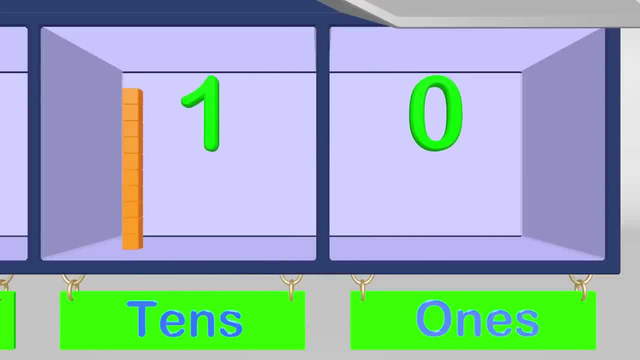 The 10s block is now in the 10s place and not the ones place. In the 10s place we are only allowed to have groups of 10.. That means we cannot have any ones blocks in this room. If we look at the number above, we see a number 1 in the 10s place and the number 0 in the ones place. 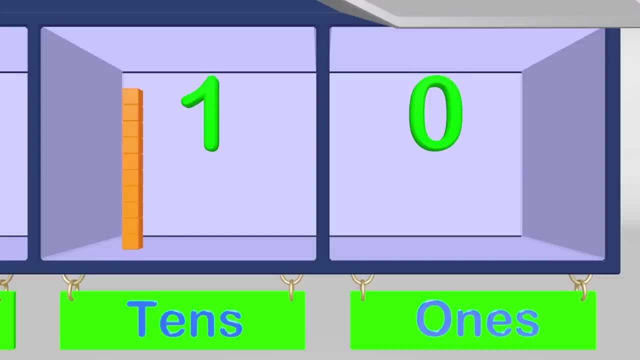 We have to remember that the 10 in the 10s place is really 10 ones blocks that have grouped themselves together to form a 10.. This is some amazing stuff to learn. Let's look at another one. Here we have 4 ones blocks and they go in the ones place. 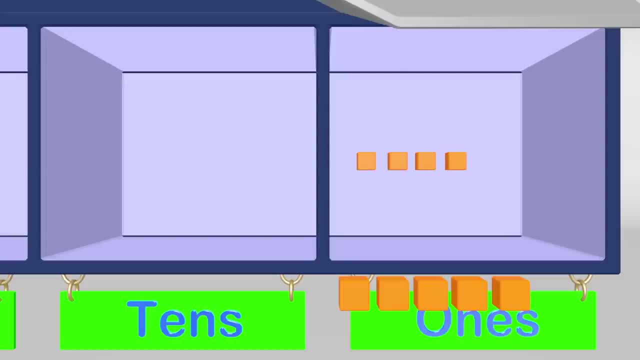 Now count with me as we add more ones blocks to the room: 5,, 6,, 7,, 8,, 9, and here comes one more. Once we have 10 of the ones blocks, we have to group them into what?